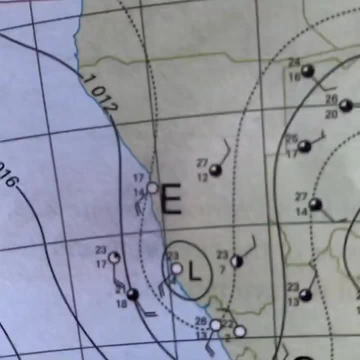 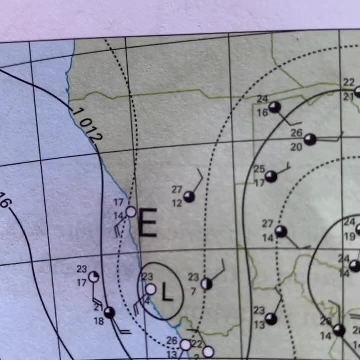 describe the weather conditions at E. So there's E, There's E okay, Okay, the yeah Okay. so, firstly, the air temperature at E is 17.. That's the one at the top, And then the dewpoint pressure. 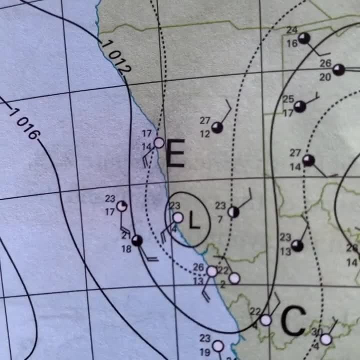 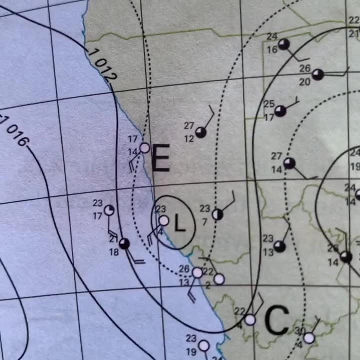 which is, I mean, dewpoint temperature at E is 17.. So that's the one at the top And then the dewpoint temperature, which is at the bottom, is 14.. The cloud cover, because that circle is empty, is clear. The wind speed: okay, the wind speed is 20 knots And for those of you who don't know why, 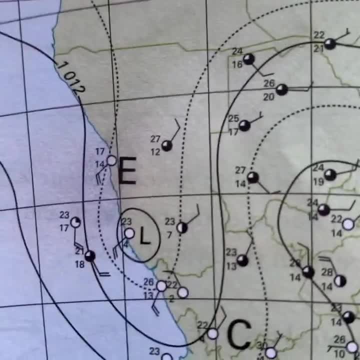 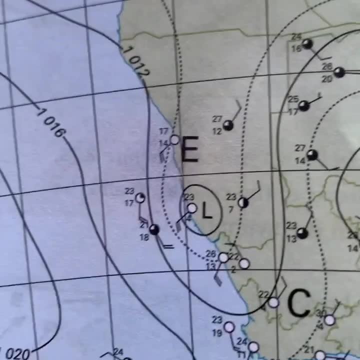 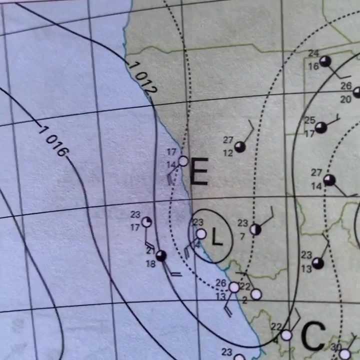 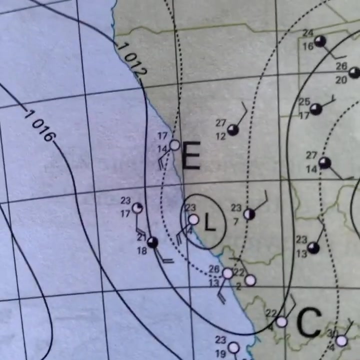 it's 20 knots, because one little line represents 10 knots And since there's two of them it would be 20 knots. And then the wind direction. I just normally draw an imaginary axis And then from that imaginary axis I find my direction, And I pre-worked this one out. 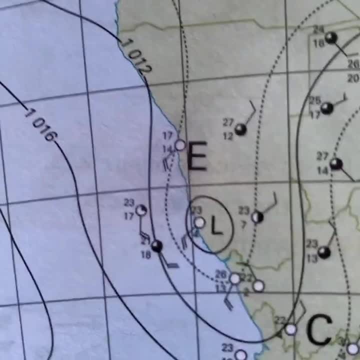 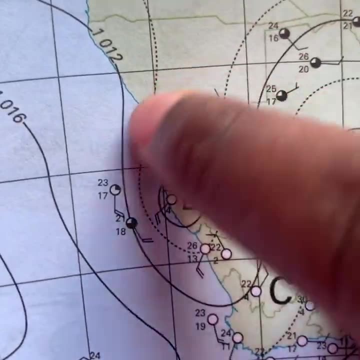 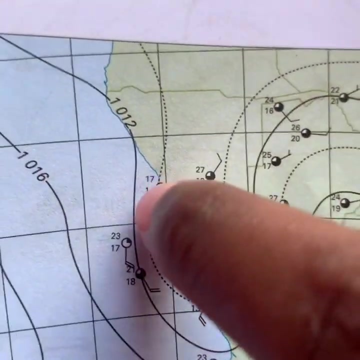 And it's west, southwest, Because, okay, I'm just gonna, it's like you draw a line there, you draw a line there, draw a line there, draw a line there And you'd see that it falls in between south and west, And then more closely to west than it is to. 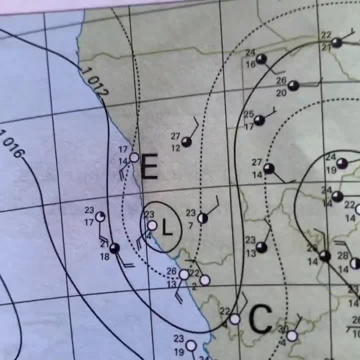 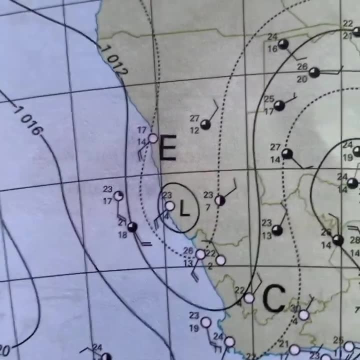 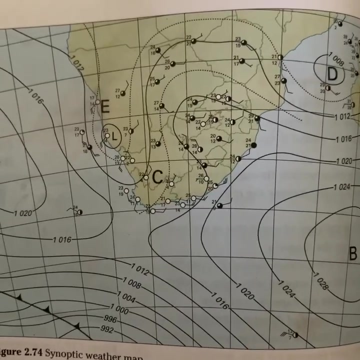 south. so that's how i got to west, south west. so, yeah, that's how you would answer the question. yeah, we've named all the characteristics. this question is out of five, so you would only need five points. so yeah, okay. so the next question says: identify the type of pressure system at f. 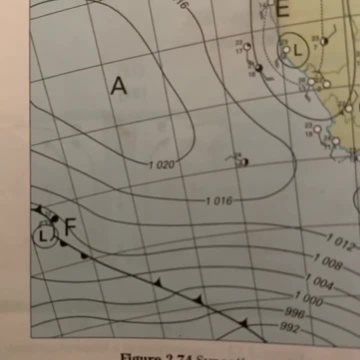 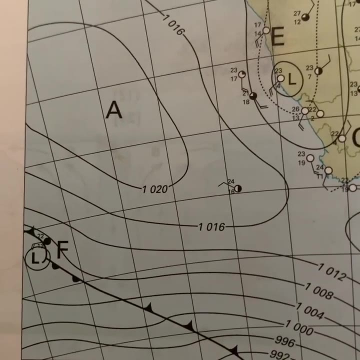 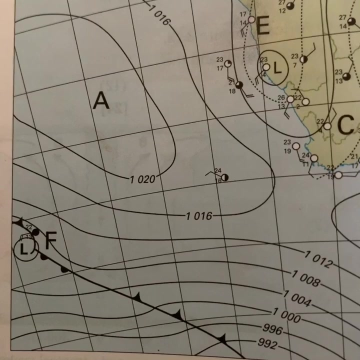 we go to f and, as you can see, there's triangles sort of, and half circles and there's a low pressure system. so if it's a low pressure and there's all these things, it definitely has to be a mid-latitude cyclone. so yeah, you just answer the question and say it's a mid-latitude cyclone. 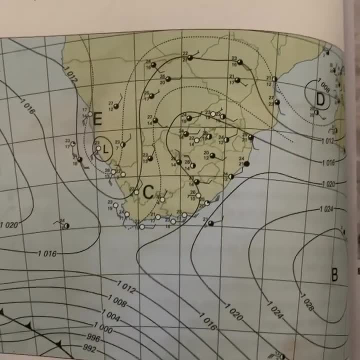 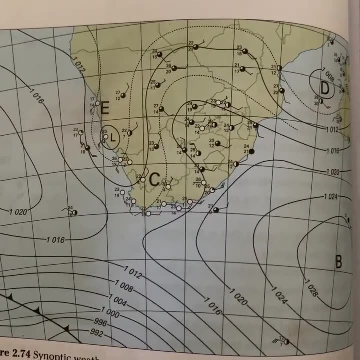 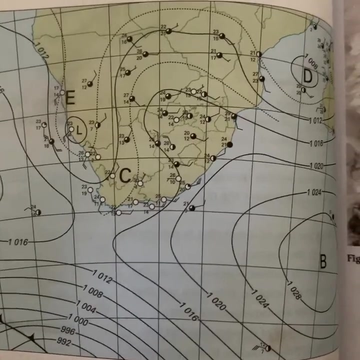 the next question. and guys, they love this question with their whole hearts, they rather love it, so they are going to be like: which season is depicted on the synoptic with a map? here's two reasons for your answer, okay. so firstly, you need to just look at what's on the 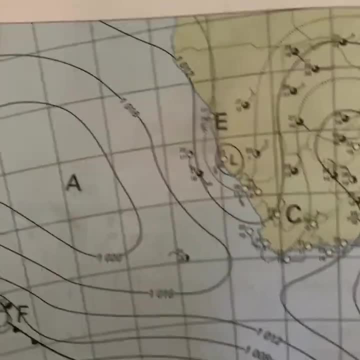 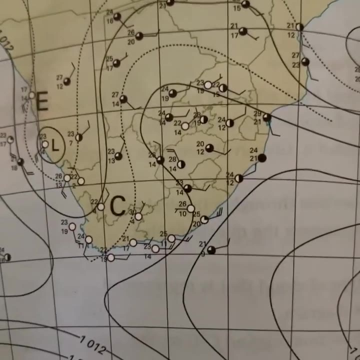 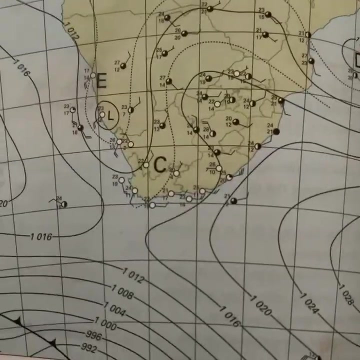 synoptic or the map. you see, there's a mid-latitude cyclone, there's these high pressure cells and also another thing that you can do is look at the air temperatures to kind of sort of give you a clue, but that's not really enough. so what i say? the answer is: it's summer. 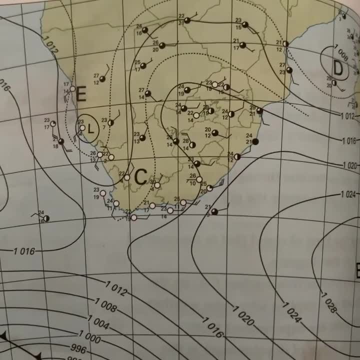 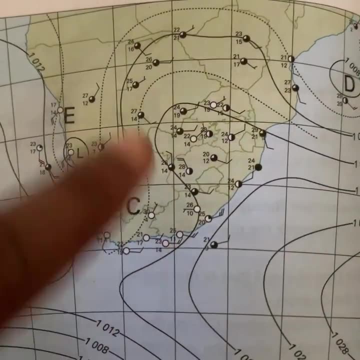 okay, the first reason why i say that is because the kalahari high pressure cell is not on the interior of south africa. had it been winter, we would have seen another high pressure cell on the interior, which is the kalahari high pressure cell. we would have seen it there. 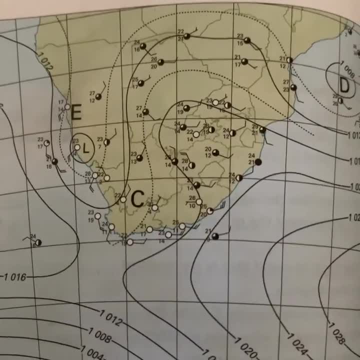 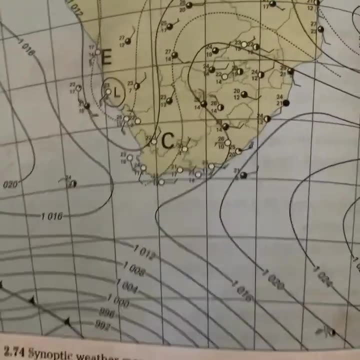 if it was winter. so in summer this high pressure cell moves downwards because of the itcz. but don't worry too much about that. but just yeah, that's the first reason. the second reason is that the kalahari high pressure cell is not on the interior of south africa. 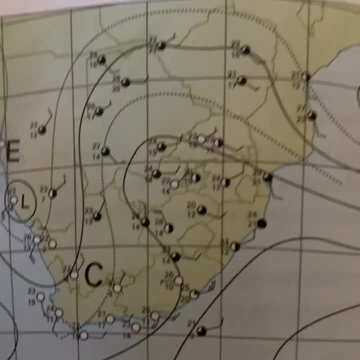 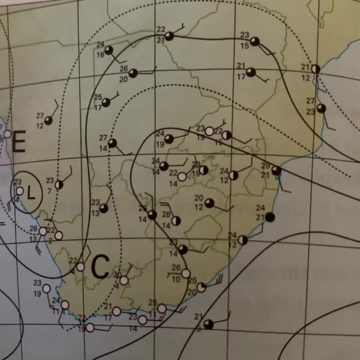 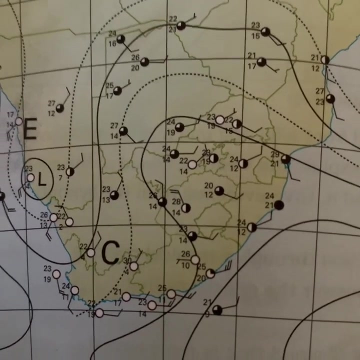 the second reason that i would give is the air temperatures. i mean, we see temperatures, air temperatures of 29, 28, 24 of 20. those are just generally not winter temperatures, those are summer temperatures. so that would be the second reason. and another reason: yeah, because you have. 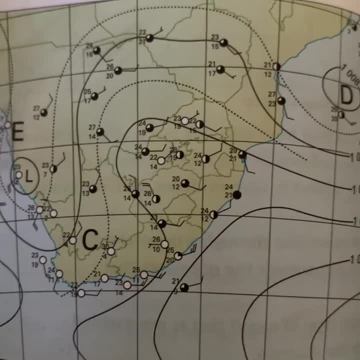 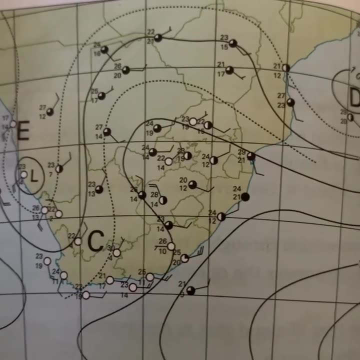 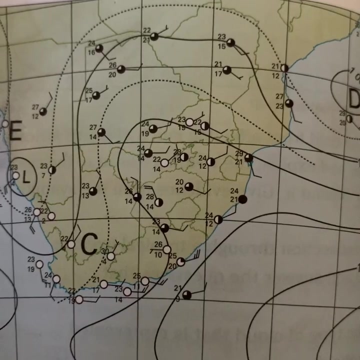 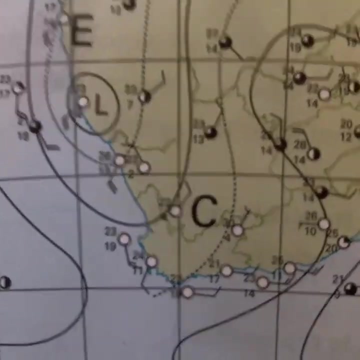 to give two reasons. so that would be the two reasons that i would give for this question. so question one point. the next question. well, it says: name the type of air circulation in the vicinity of sea and explain why it might cause a fire hazard. okay, see, see, it's there, the air. 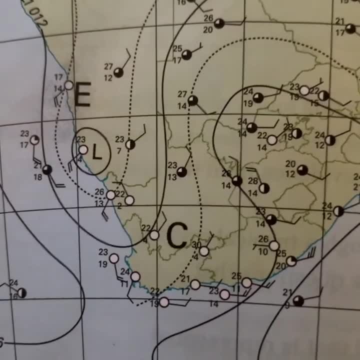 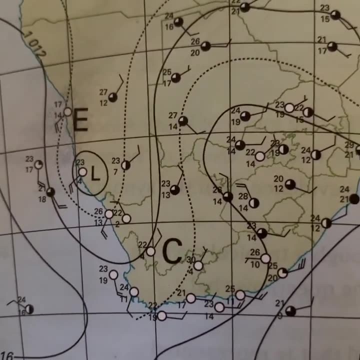 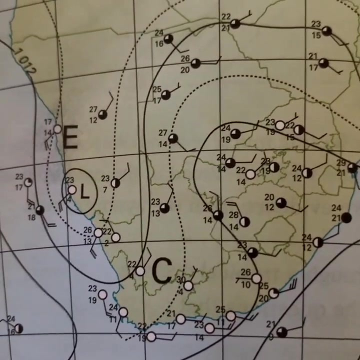 circulation of c would be um anti-clockwise, because sea should be a high pressure cell. therefore, C is there. air東이 should flow from the top to the rim, sm Инfrared water valve x to the bottom. therefore, as it flows from the top to the bottom, it's gonna heat up adiabatically. 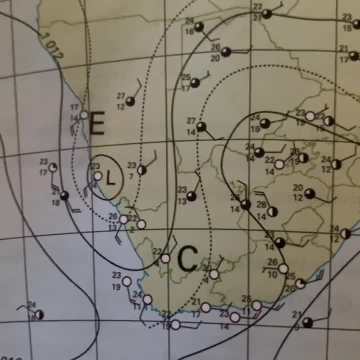 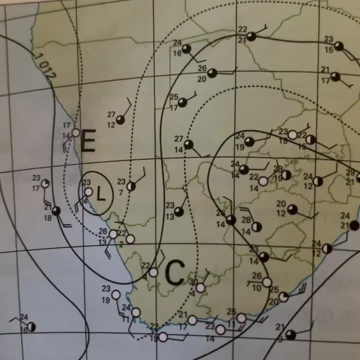 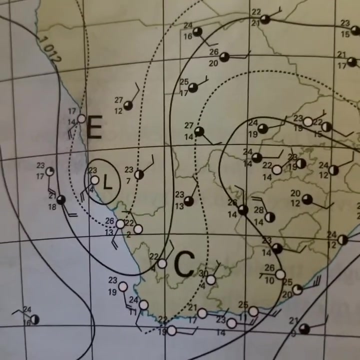 so that is why it might cause a fire hazard, because it's dry air as well. so this dry air, as it flows downwards it gets hotter and hotter and hotter, and if it finds no moisture on the ground, it's like dry and everything. it might cause a high hazard because it might start fires. 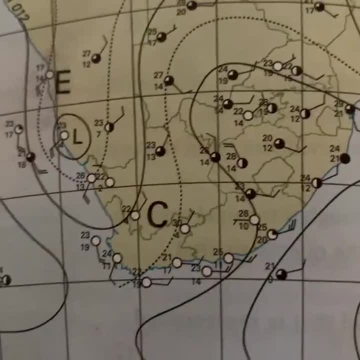 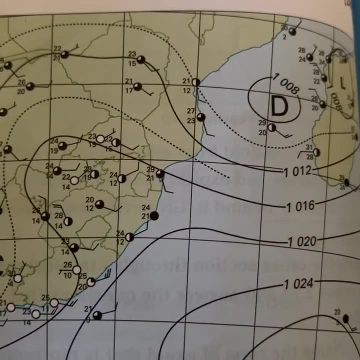 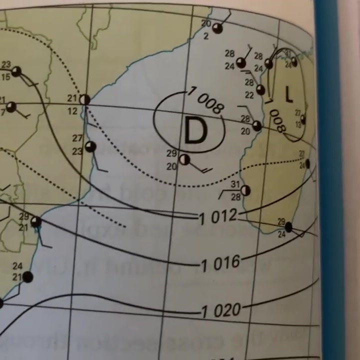 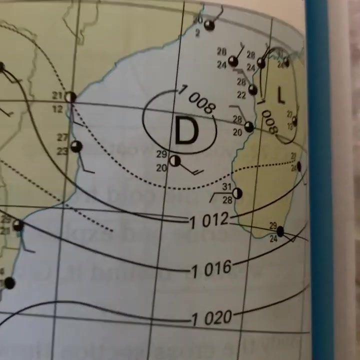 so that would be what i would answer. and then 1.7 says an amateur with a forecaster predicts the development of a tropical cyclone in the area at d, which is there. do you agree with this prediction? explain your answer. yes, i agree with this amateur weather forecaster. okay, firstly, 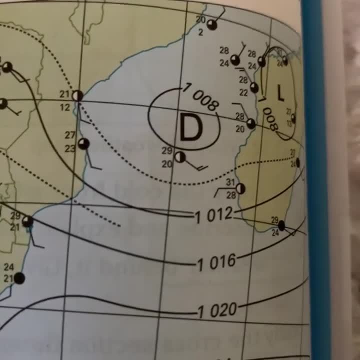 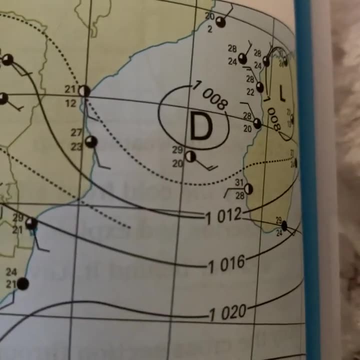 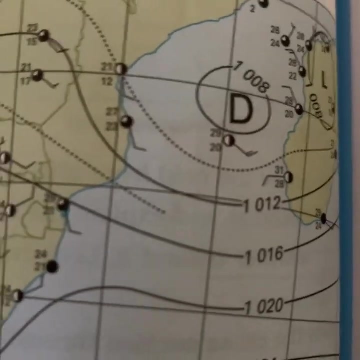 we see from the weather station at d is that the air temperature is 29 and, as you learned earlier, is that um for the development of a tropical cyclone, the it's in the, the temperature of the water should be greater than 27 degrees. well, it is here. 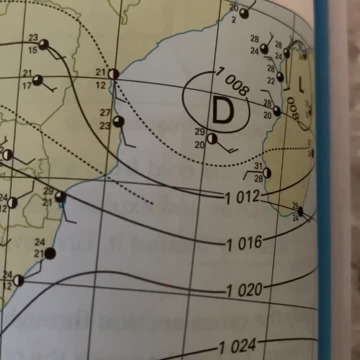 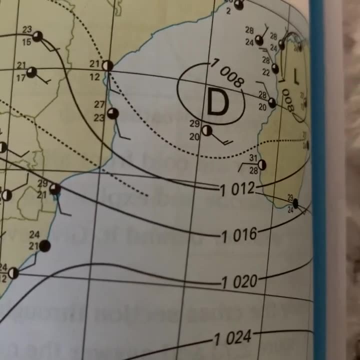 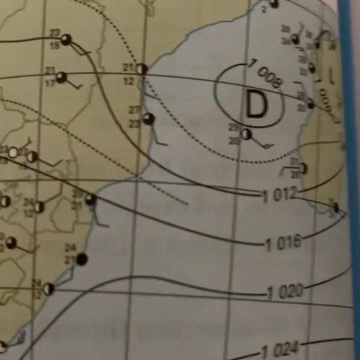 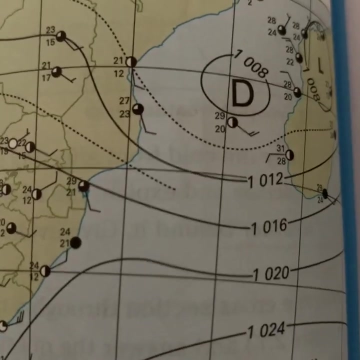 as we see it. secondly, that pressure, it's 1008, which is mostly the pressure that you find um, when the, when a tropical cyclone reaches the immature stage, and stuff like that, so that air pressure is that of a a tropical cyclone. so i agree with him, okay. other reasons: well, the location. 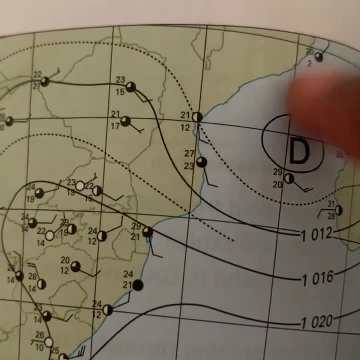 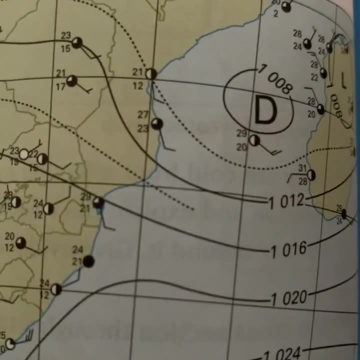 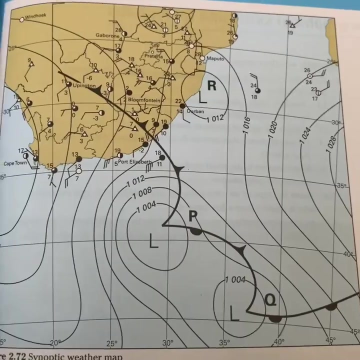 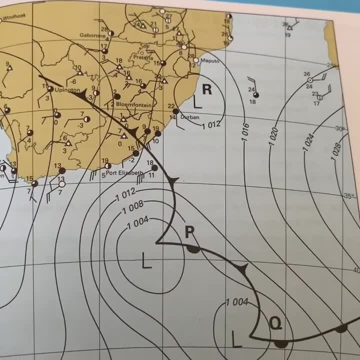 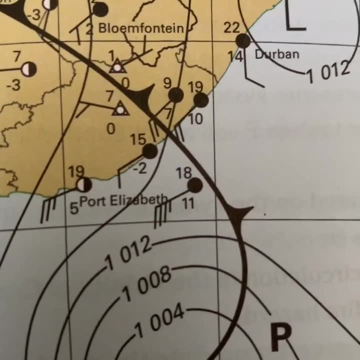 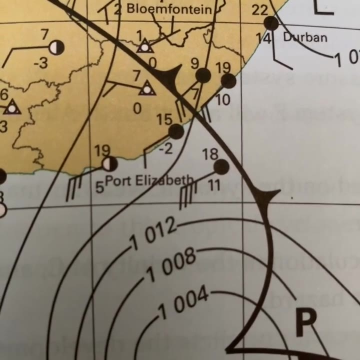 first question would be describe the weather at port elizabeth. so we zoom in, we go to port elizabeth, we look at that weather station. the air temperature which is at the top, 19 degrees. the dew point temperature which is at the bottom is five degrees. the cloud cover is half as 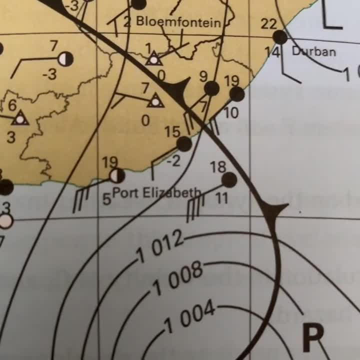 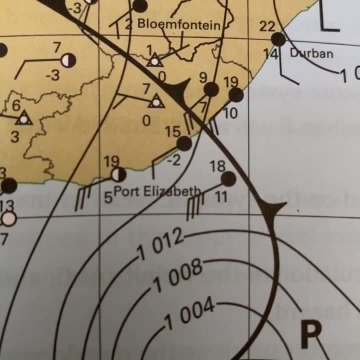 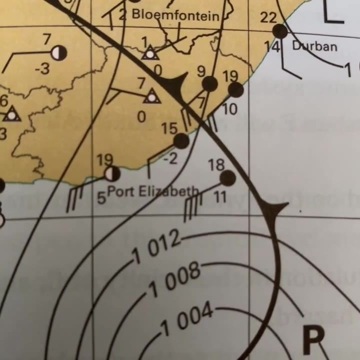 indicated by that circle, so only half of it is shaded. the wind speed: oh wow, that is hectic. so the wind speed is 25 knots, and the reason why i say it's 25 knots is because there's two, two full ones and one half. one and a half represents five, so the wind speed is 25 knots. 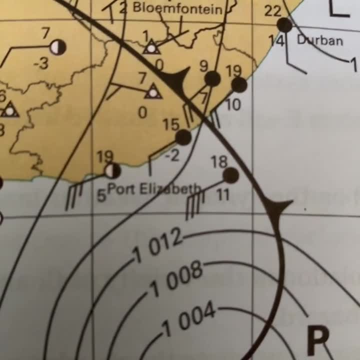 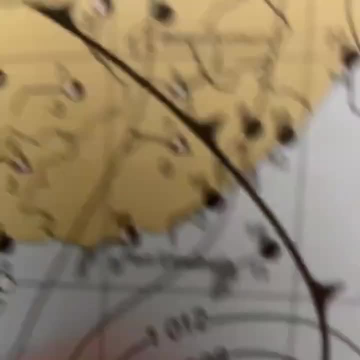 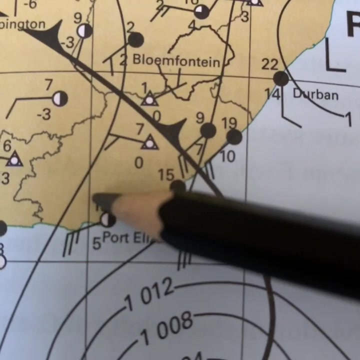 guys, that is really quick, i mean fast, that is really fast. and then the direction. okay, i just have to just work this out, because it's not really something that i can just see from the top of my head. okay, so i'm going to draw my imaginary axis again. 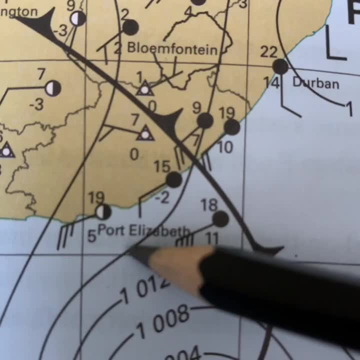 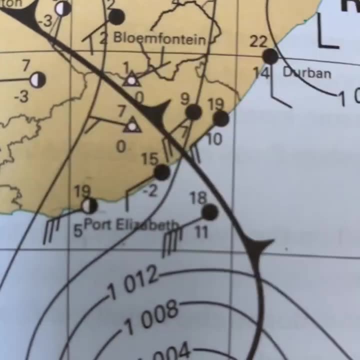 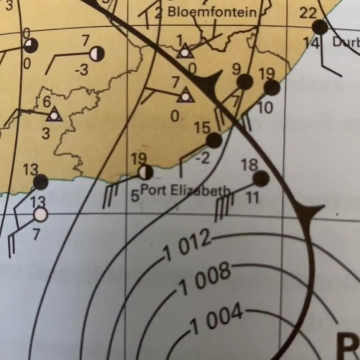 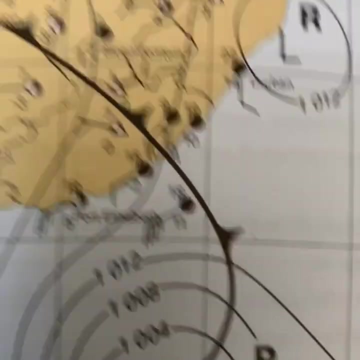 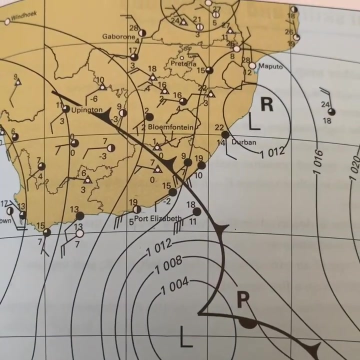 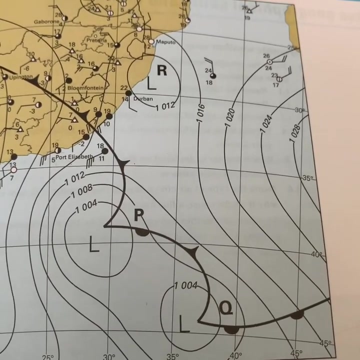 nope, wait. no, that is definitely um west southwest. so okay, that wind direction is west southwest. so yeah, that is the weather at port elizabeth. oh, my word, i feel like a weather lady. okay, name the weather features at p and q. p and q, the weather features okay. p because they are triangles. 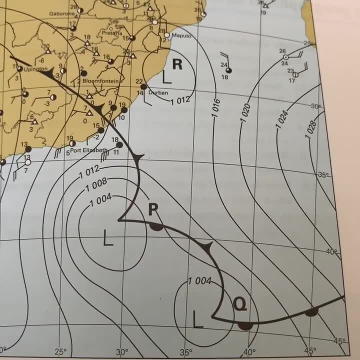 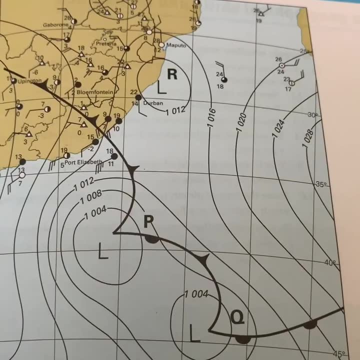 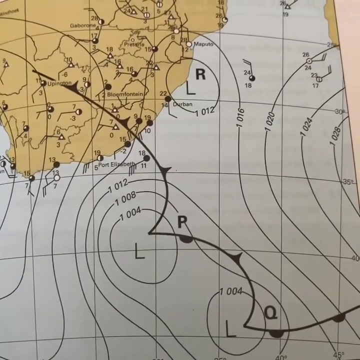 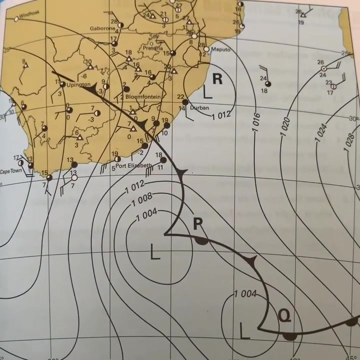 that would be the cold front, and q, because they are half little circle thingies, that is the warm front. so yeah, the next question says: in which direction? oh, sorry a fan, in which direction are p and q moving? as you know, um mid-latitude cyclones move from west. 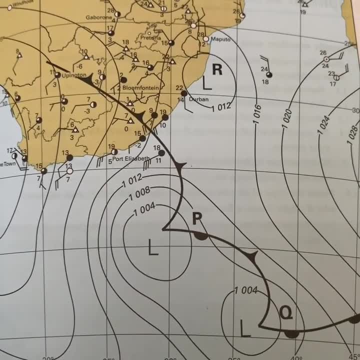 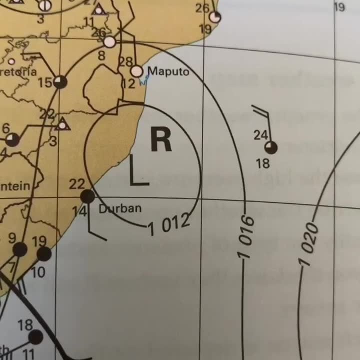 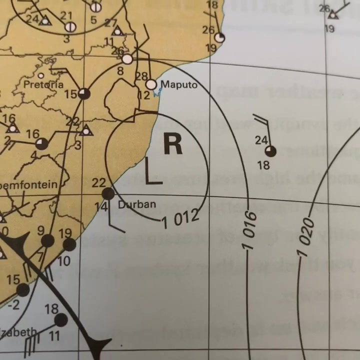 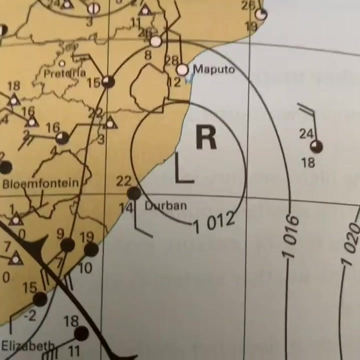 to east so we can say that they are moving in an easterly direction. name the weather feature at r: r, that is a coastal low. yeah, that is a coastal low. it occurs at the coast and it is a low pressure. solve okay. and the next question says: how is r affecting the weather at durban, while r seems to have kind? 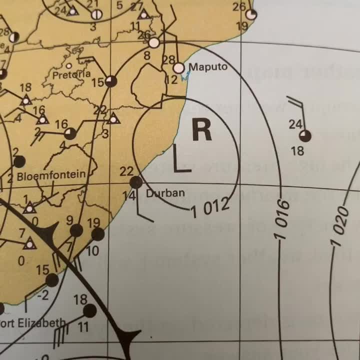 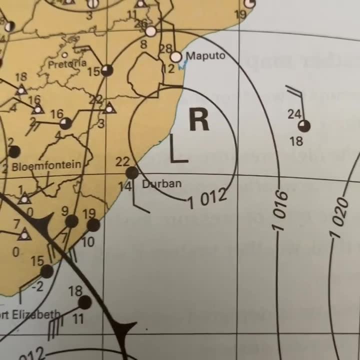 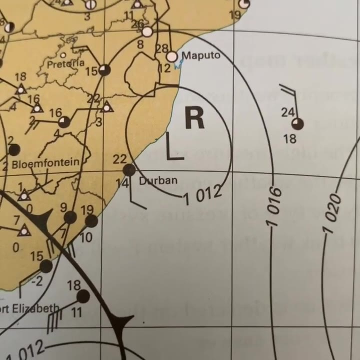 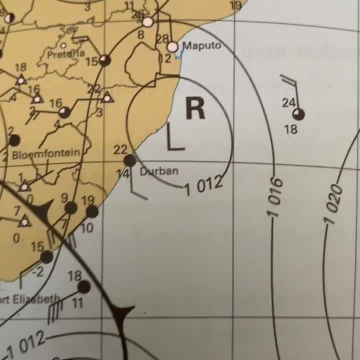 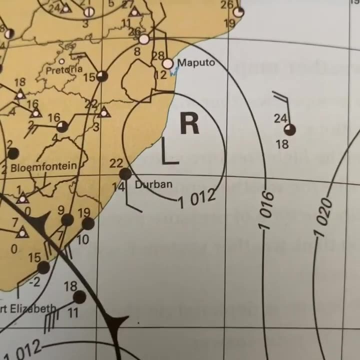 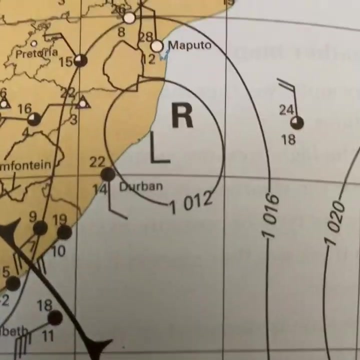 windy. so a coastal low does that. after it's past a region like the area becomes cold, comes windy, becomes very wet. so yeah, that's basically how you would answer that question. well, not really, because they just asked how it's affecting the current weather. so you would say it's cloudy because you 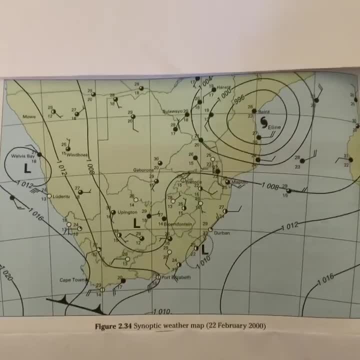 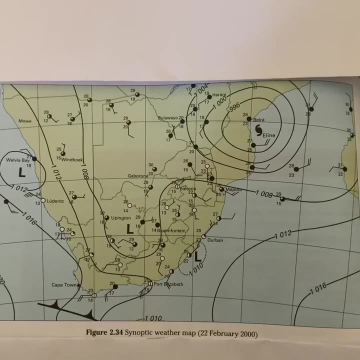 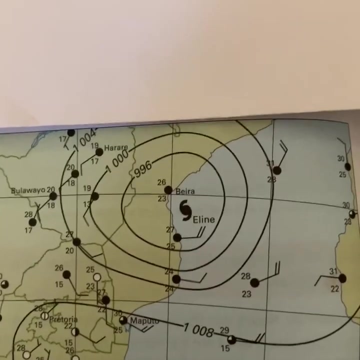 can see that it's overcast. okay, here is another synoptic weather map. so the first question says: give four reasons why you know the pressure cells are overcast and the temperature is too high and the protective AC CHR zone that's centered at bay area is a tropical cyclone there. that one, okay. so 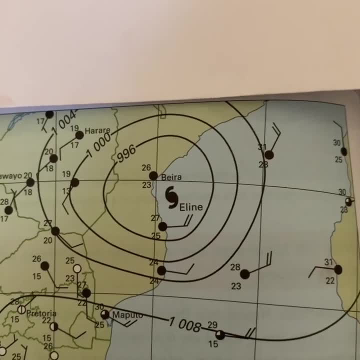 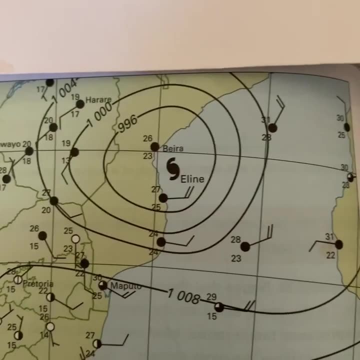 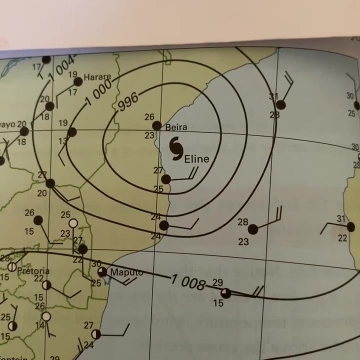 the first reason would be, firstly, the name. only tropical xyclones have names, not mid latitude cyclones, not high pressure styles. only tropical cyclones have names. so that's the first reason. the second reason is the air pressure. the pressure is pretty low and it's steep. 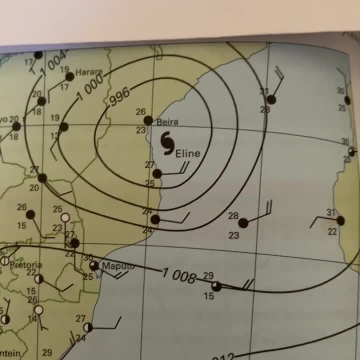 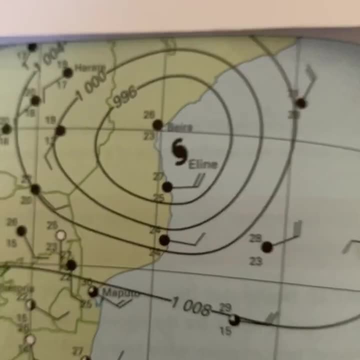 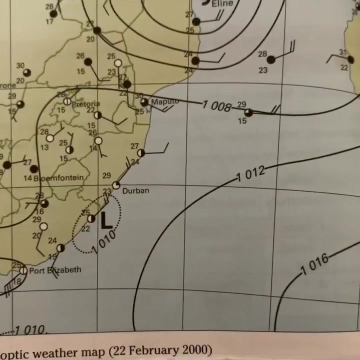 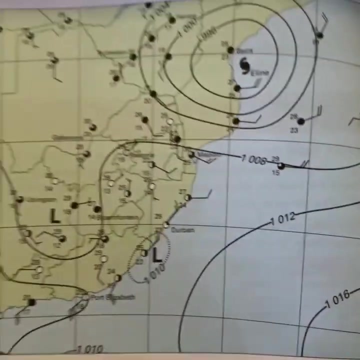 excuse me quick and fast, the. the decrease is pretty steep. so that would be the second reason. the third reason is that symbol there at the eye. so that's the second reason, oh, my word. and then the fourth reason. they gave us such an amazing clue. they gave us this date, which is 20, 22 february 2000, and as 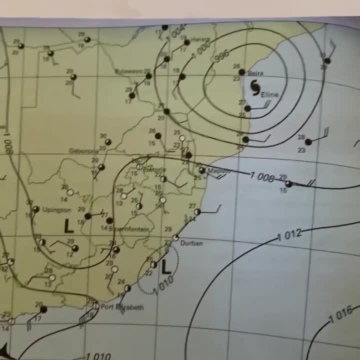 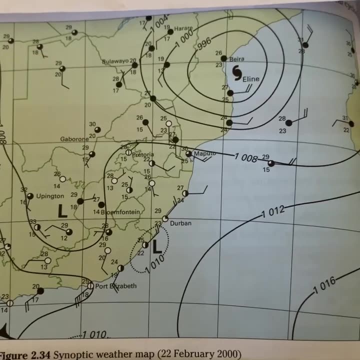 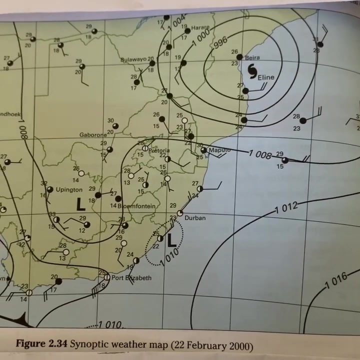 you know, a tropical cycle happens in late summer, early autumn and in the southern hemisphere, like, 22nd of february is towards the end of summer and the beginning of autumn. so those are the four reasons that tell us that that is a tropical cyclone. describe the weather conditions. oh, my word. 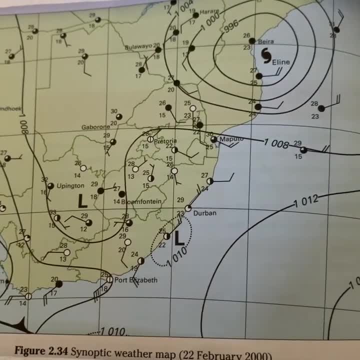 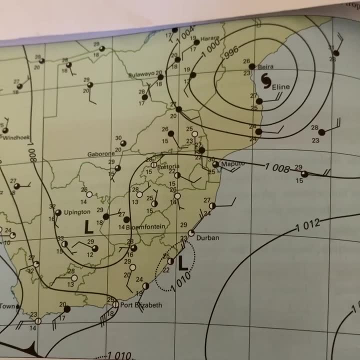 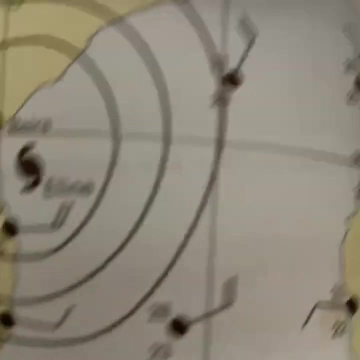 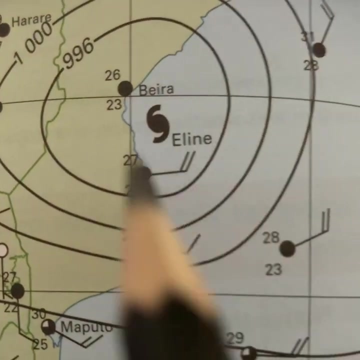 not again, but yes, this question they always ask: describe the weather conditions, pressure, temperature, clouds, winds and rainfall associated with cyclone line or elene, as shown by the weather stations on the map. okay, i'm gonna zoom in too. okay, so we have to. okay, i'm just gonna do this one. yeah, this one. 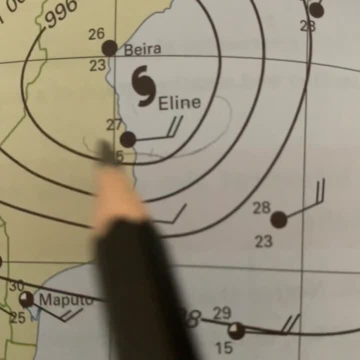 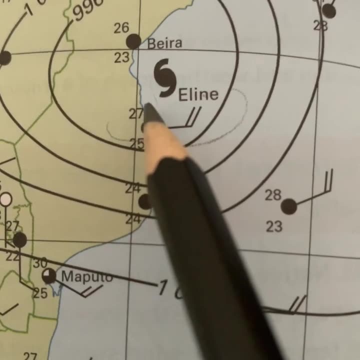 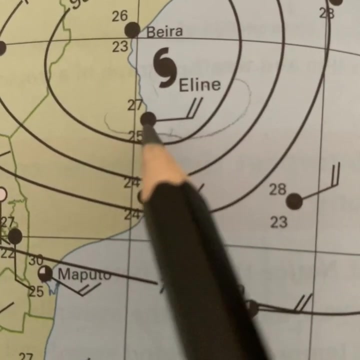 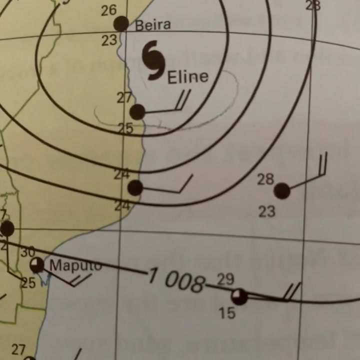 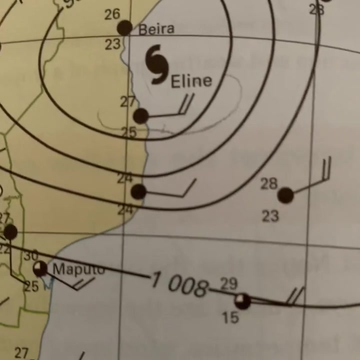 because it's closer to there. okay, so, firstly, the cloud cover, overcast air, temperature: 27 degrees, do you point? temperature: 25 degrees. the wind speed: 20 knots. the wind direction: that is definitely east. yeah, that is east. and then what else did they say pressure: okay, we've done rainfall, okay, although. 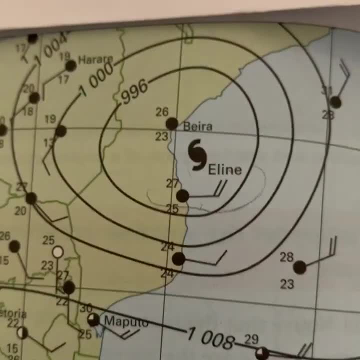 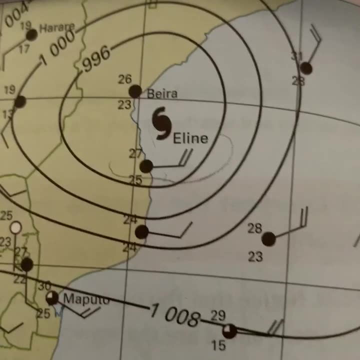 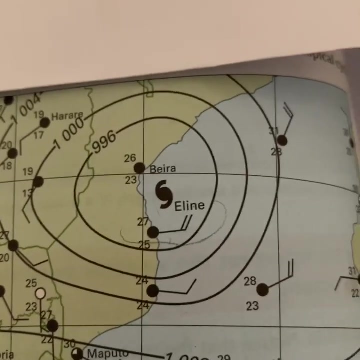 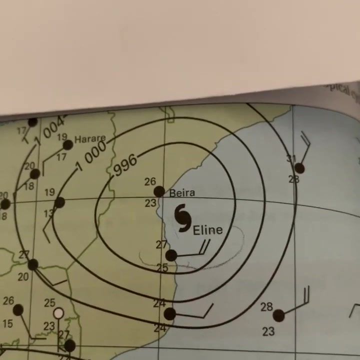 there is no symbol of rainfall, but you know that because it's a tropical cyclone, there are thunderstorms and yeah, and because it's it's in the mature section sector, i mean, of the tropical cycle, i would say there's thunderstorms and then, even though they didn't put a symbol, but yeah, and then the air pressure is 996, so we have. 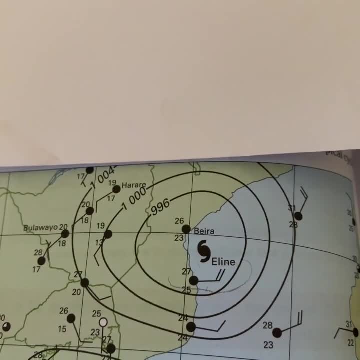 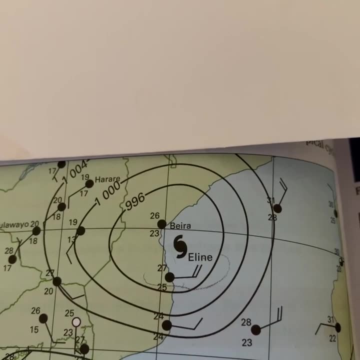 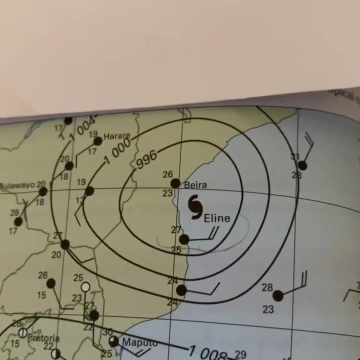 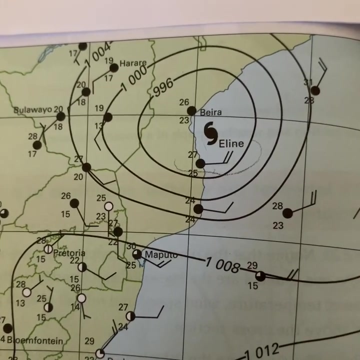 answered that question, um, the next question would is: what stage of development is cyclone in line? motivate your answer: go answer, go, go answer. okay, let's get serious. the stage of this tropical cyclone is the immature stage, and the reason for this is that the the lowest air pressure is 996, so that would definitely. be immature because had it been in the mature stage, the lowest air pressure would have been lower than 950. so yeah, that is why i say it is in the immature stage, okay. the next question says: predict what will happen to cyclone elian in the days following this one. well, the cyclone. 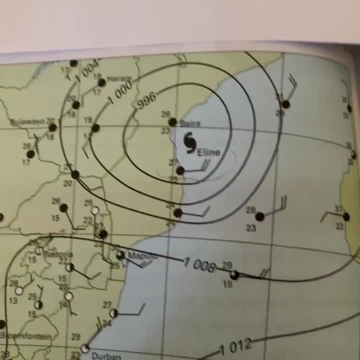 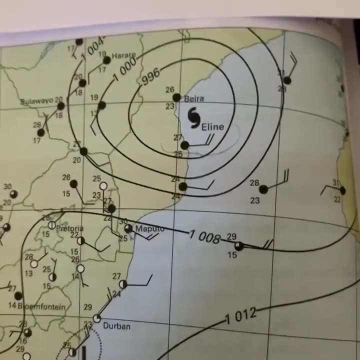 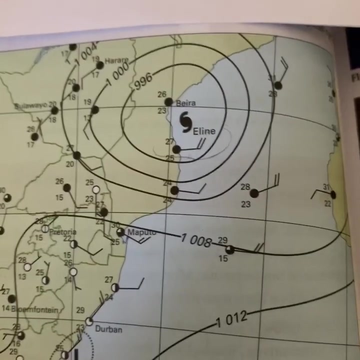 is getting closer to land. so okay, because it's still in the mature stage. it's still going to be in the mature stage, so wind speeds are still going to increase, the the air pressure is going to decrease even more and there's going to be a clear, clear eye and 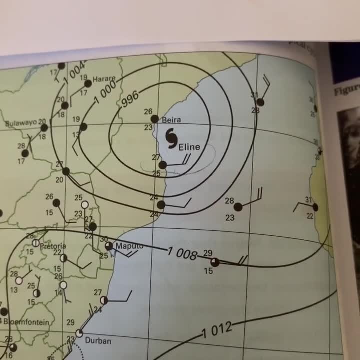 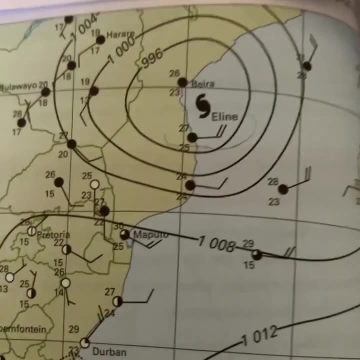 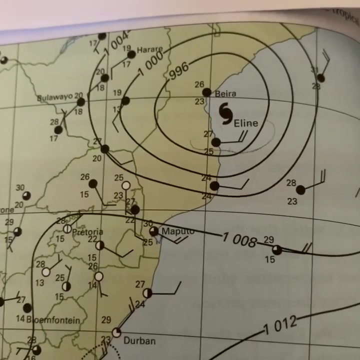 where there's a clear eye. the conditions are going to be cloudless, they're going to be clear, it's going to be sunny, there's going to be no rain, and so, as it moves towards the land, it's going to start to degenerate because of the friction on the land, and a and tropical cyclones don't. 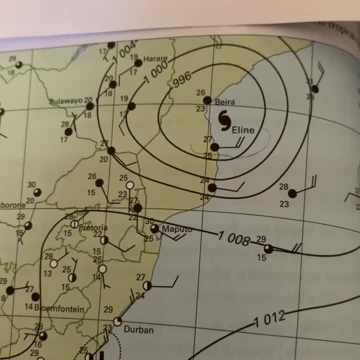 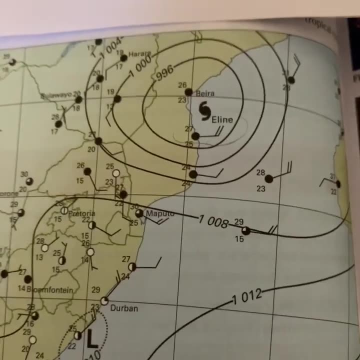 is it safe to say they don't like, yeah, they don't like friction. friction like causes them to die out. so that's what's going to happen. and yeah, and it's going to go back to sea. so that's what's gonna happen. okay, guys, so that's. 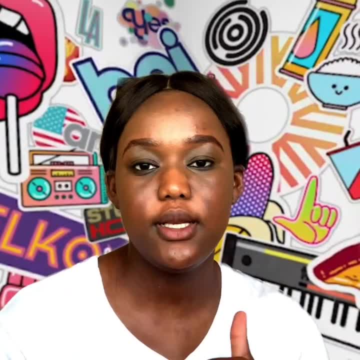 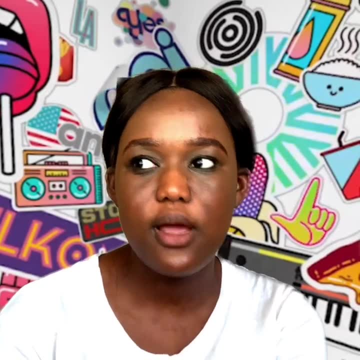 it for today. synoptic weather maps done. um, i would advise you to go practice more past papers and i mean, if you have any questions, i'll be more than willing to help. just drop a comment on the comment box and just say if you have any questions, just drop a comment on the comment box and just say.